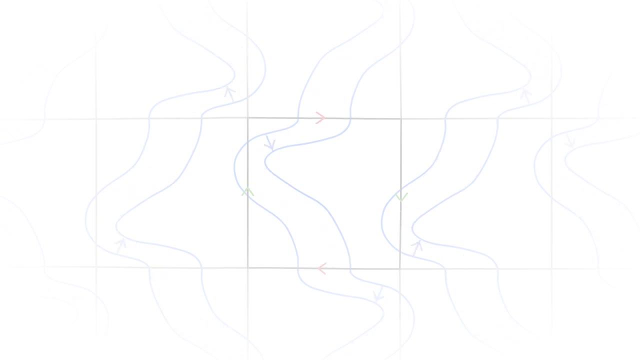 as it may seem Now. unfortunately, algebraic topology is not the only way to invent homology. It's also one of the ways to invent it, but not the only way to invent it. Topology has a lot of prerequisites, But in this series I'll be talking mostly about ideas, and I'll 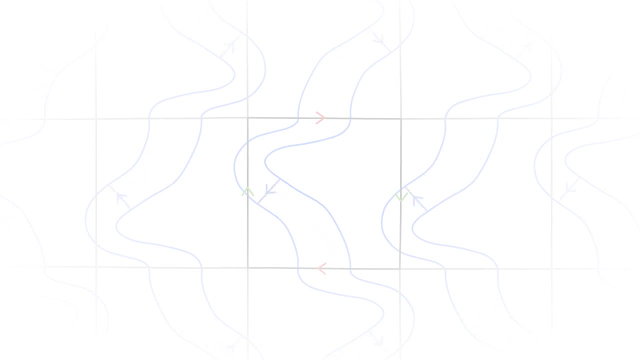 push back the prerequisites as far as possible. I will eventually have to assume that you know some group theory and so on. but I'll wait as long as possible and it's my hope that if you don't know any group theory, all the stuff up to that point will be clear. 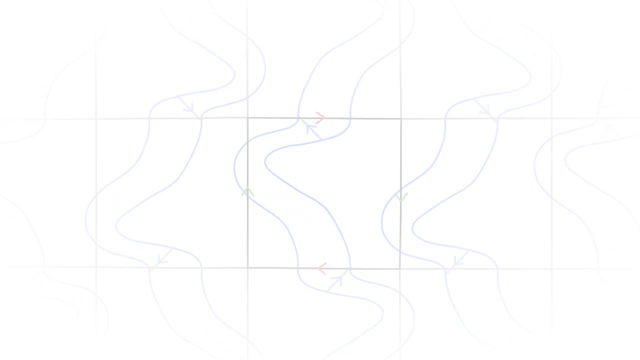 After all, the algebra, in algebraic topology, is largely a bookkeeping device and the ideas that the groups formalize exist independently of the groups themselves. So every video will have very clearly stated prerequisites at the start. The first video, which provides a philosophical background and motivation. 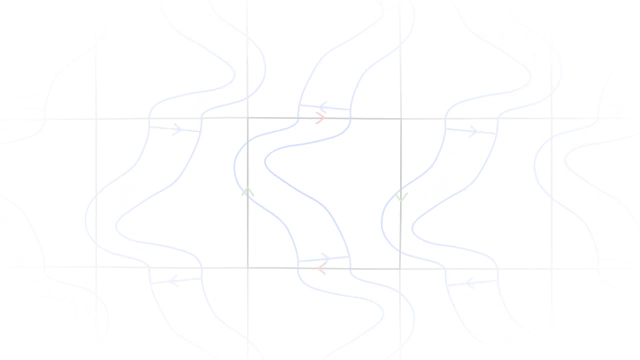 doesn't have any specific prerequisites besides knowing what a function is, and even that should hopefully become clear during the course of the video if you're unfamiliar. So anyway, thanks for watching, like and subscribe, and let's get to the content. 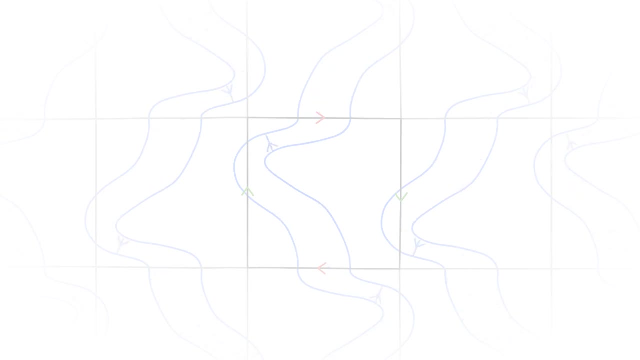 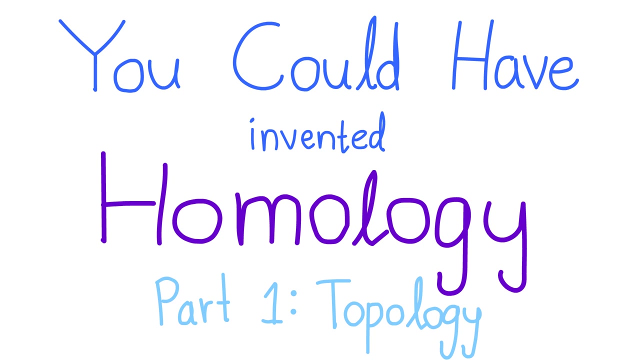 Oh, and just as a heads up, I will be using the words function, map and mapping interchangeably throughout. Topology is the study of continuity. Continuity is a property that functions can have, and it really is a thing. Typology is the study of continuity. 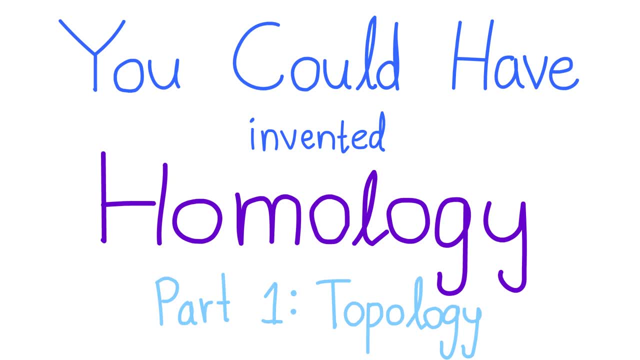 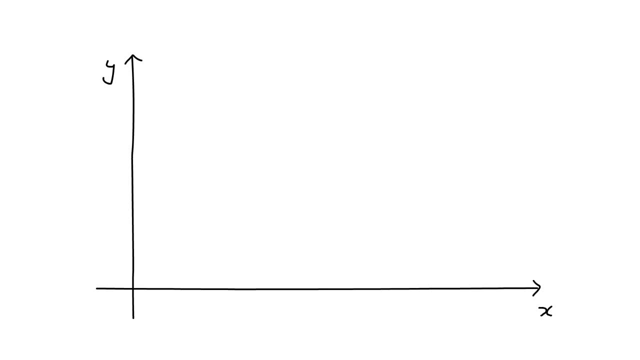 It is a property that functions can have, and it really is a thing. And it really is a thing roughly means that the function doesn't tear its domain. For instance, a function from the real line to itself is continuous when its graph can be drawn without lifting your pen from the page. 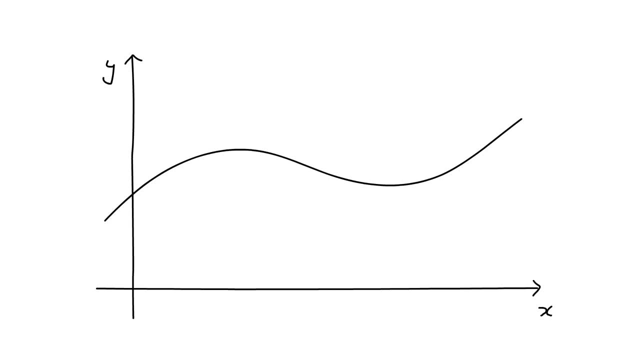 If we think of the graph of this function as a sort of distorted copy of the line, then the function is continuous when its graph is still a line. It may be bent or curved, but it's not broken. Another way to think about continuity is that a function is continuous. 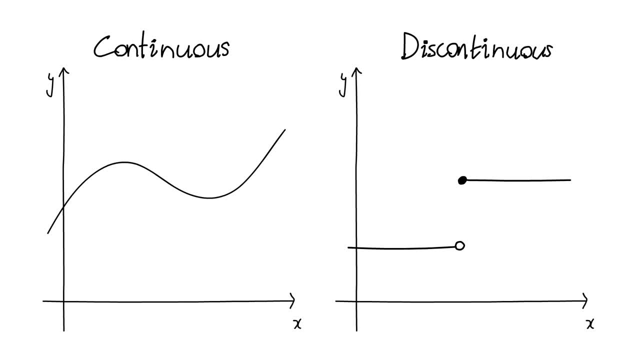 when it sends nearby points to nearby points. If we pick a point in the domain of a continuous function and wiggle it a little, then the corresponding point in the codomain can move, and maybe it can move a lot, but it can't suddenly jump. 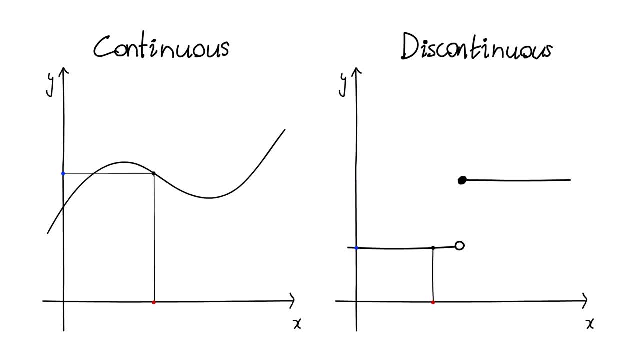 Continuity is an important and pervasive concept in mathematics and lots of geoscience have shown it. Geometric and even not-so-geometric things have some notion of continuity. For instance, we can talk about whether or not a function from a line to a plane is continuous. 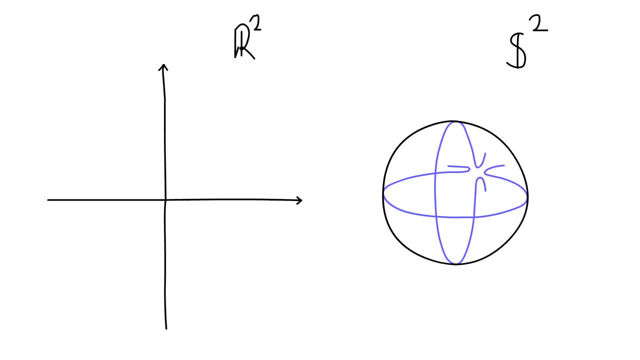 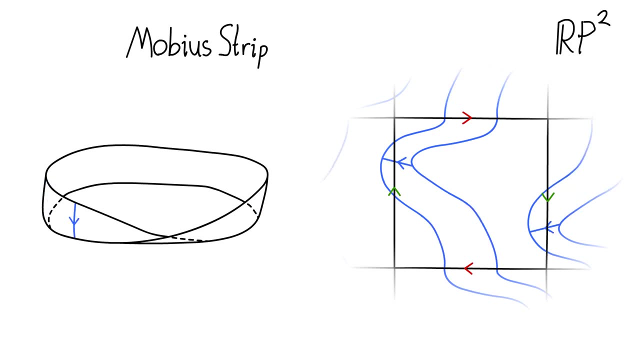 or whether a function from a plane to a sphere is continuous, or really any function between any two things that are in some sense spatial. In fact, having a notion of continuity is arguably what it means, or what it means, to be a function, Or at least part of what it means for something to be a space. 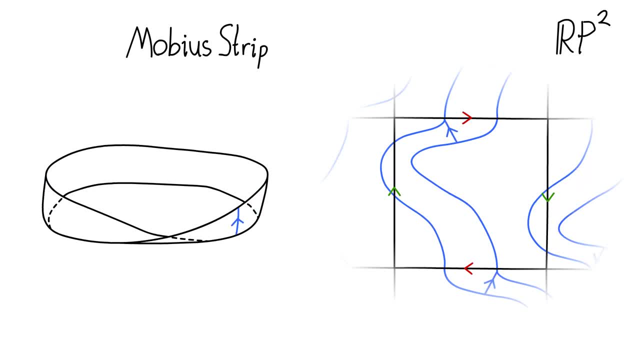 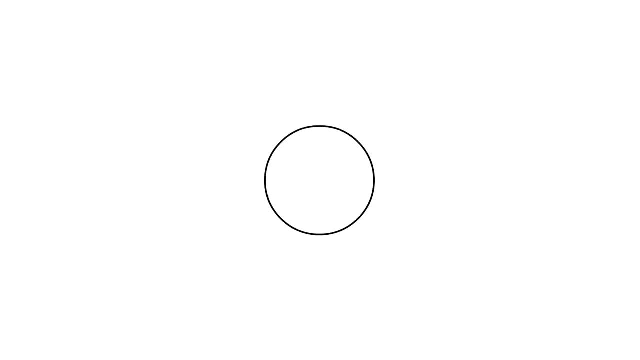 In topology, the main objects of study are called topological spaces. Topological spaces consist of a set of points together with some notion of continuity. A notion of continuity in this case comes in the form of a mathematical gadget called a topology, that determines which functions mapping out of or into the space. 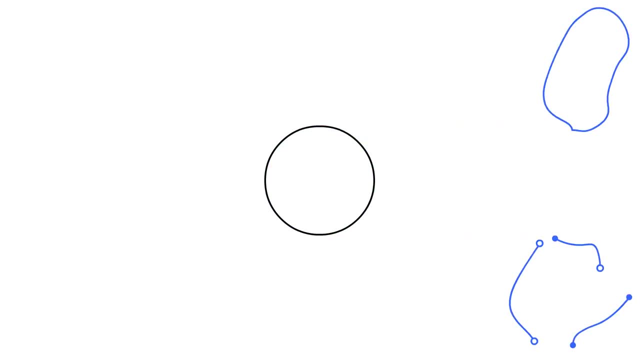 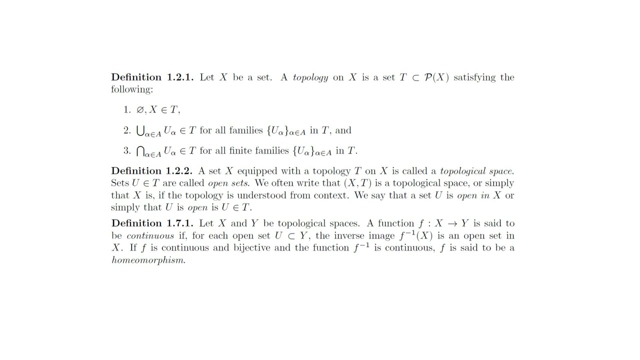 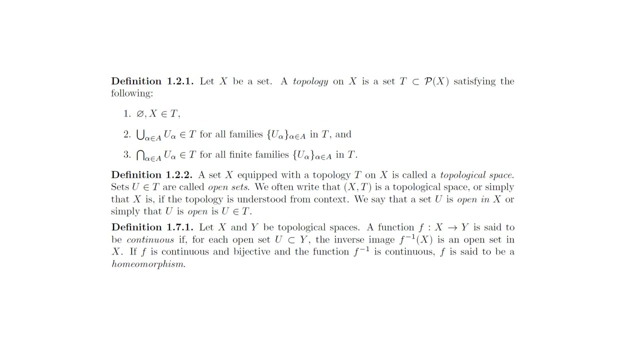 are continuous So long as the other set involved also has a topology. The technical definition of what a topology is is a bit unintuitive. I don't think it would be a helpful digression to go through the nitty gritty details of what a topology is and how the continuity gadget works. so I won't, although I may make a video. 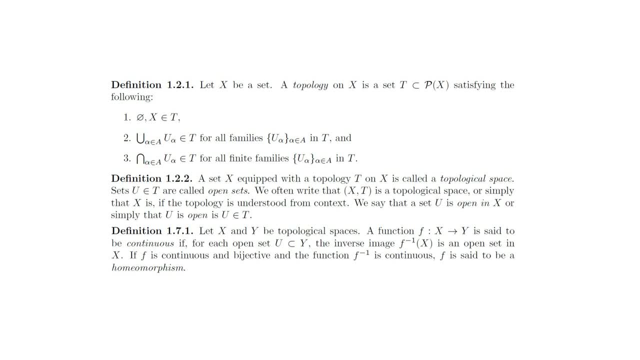 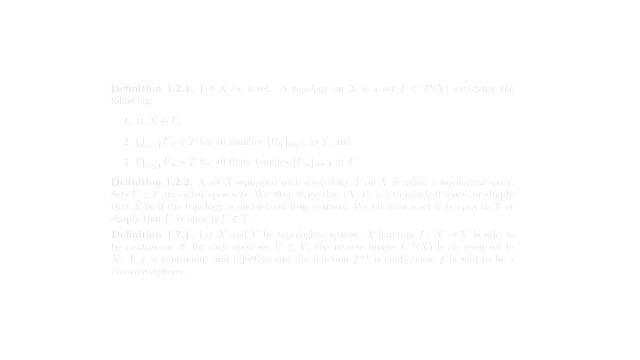 about it in the future. But now just think of it as a topology. Think of it as a machine that says yes or no whenever it's given a function and another topology to compare notes with. The goal of topology is to understand topological spaces. 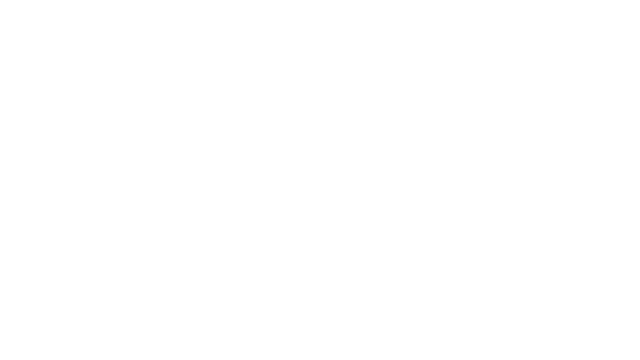 Since topological spaces show up all over mathematics, topology has grown to be one of the central topics in modern mathematics. So what does it mean to understand topological spaces? Well, ideally we'd like to write down a list, a so-called classification, of all the 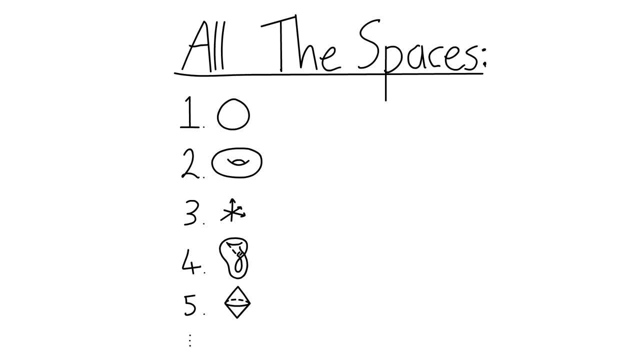 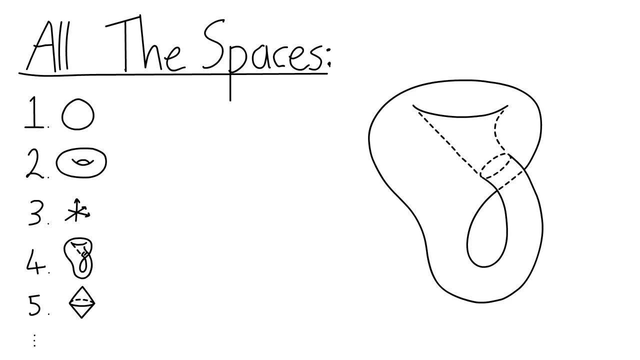 topological spaces that can possibly exist. Then whenever a topological space pops up, as so often happens in mathematics, you can ask: which topological space on our list is this? A good classification would come with a way to figure that out. and if we had such a classification? 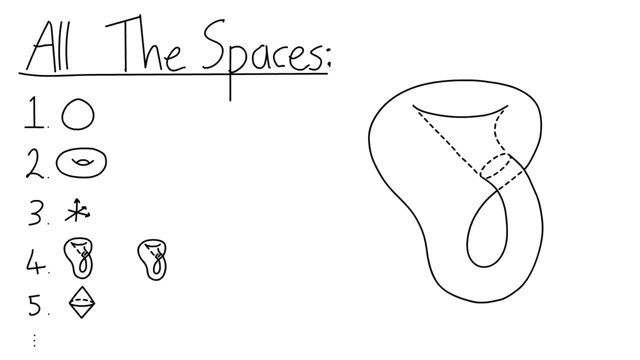 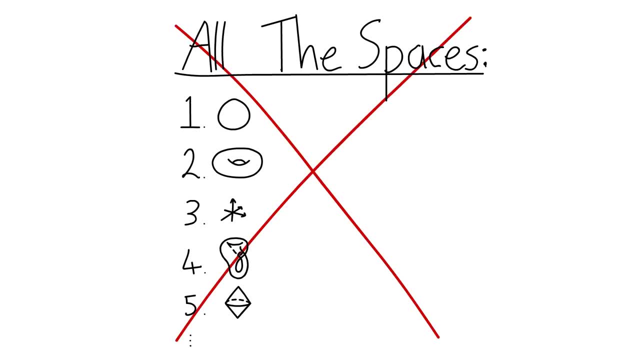 we would have to know an enormous amount about topological spaces. Unfortunately, classifying topological spaces is extremely impossible. The universe of topological spaces is so expansive that not only would it be astronomically impractical, you can even prove that it's impossible. 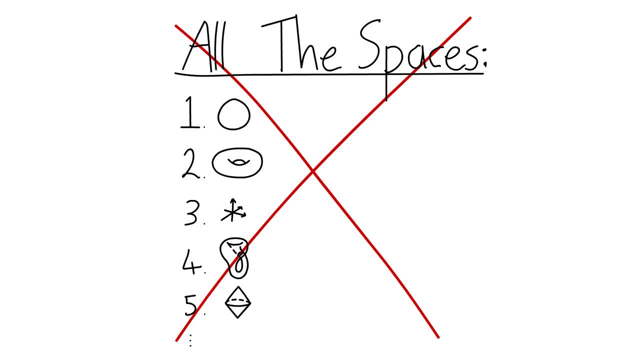 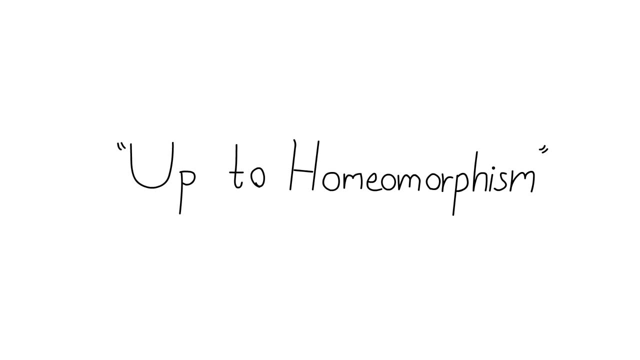 We can somewhat reduce the number of topological spaces we have to study by considering the topological spaces. What does that mean? Well, some continuous maps don't really do anything. Consider the following mapping: from this torus to this coffee mug, There is another continuous map which goes the other way. that undoes our map in the. 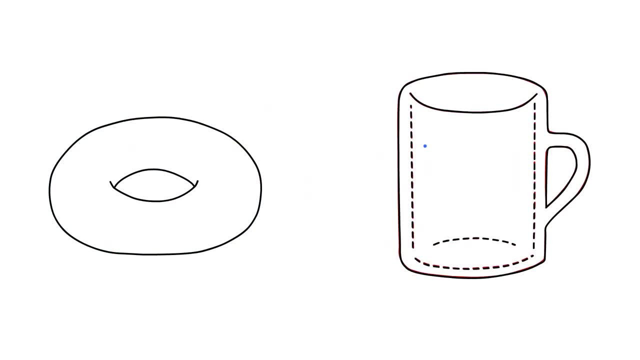 sense that if you apply one and then the other in either order, you always end up back where you started. So this map can't really change anything about the Taurus, at least nothing that you can't undo by applying another continuous map. This means that the Taurus and Coffee Mug have to have essentially the same shape in 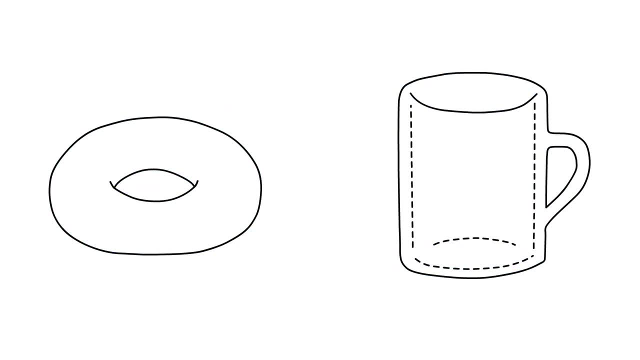 a very loose sense. After all, you can turn one into the other by a reversible, continuous transformation In topology. we call reversible continuous maps homeomorphisms, and if two spaces have a homeomorphism between them, we say that they're homeomorphic. 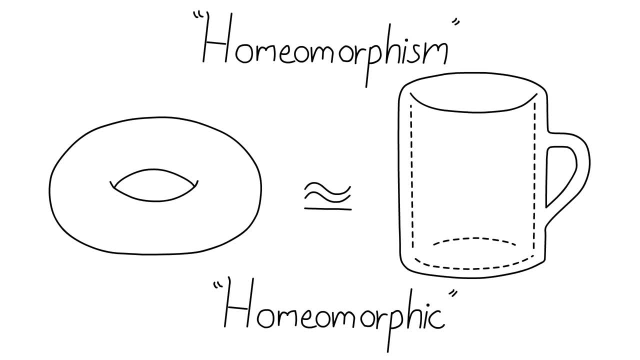 Homeomorphic spaces are thought of as being basically the same, at least as far as topology is concerned. Studying topological spaces up to homeomorphism then means studying topological spaces while disregarding any difference between homeomorphic spaces. This is part of a wider theme in mathematics, when you want to compare objects or tell 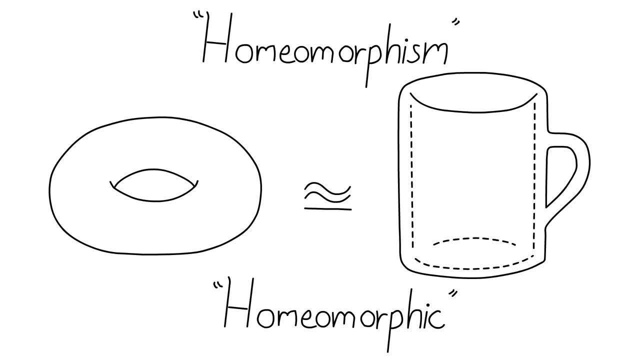 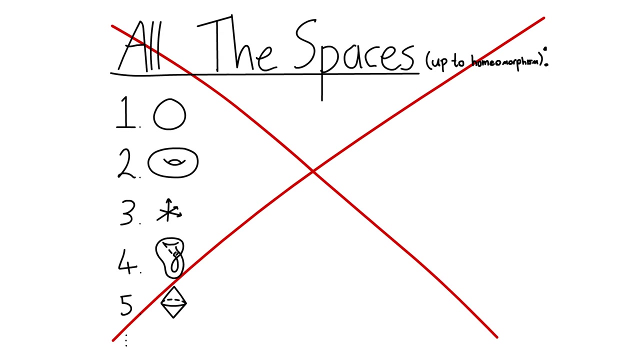 them apart by detecting some fundamental and intrinsic difference. transformations that can be undone are thought of as doing essentially nothing, and objects that can be turned into one another are thought of as doing essentially nothing. Unfortunately, it's still extremely impossible to classify topological spaces, even up to